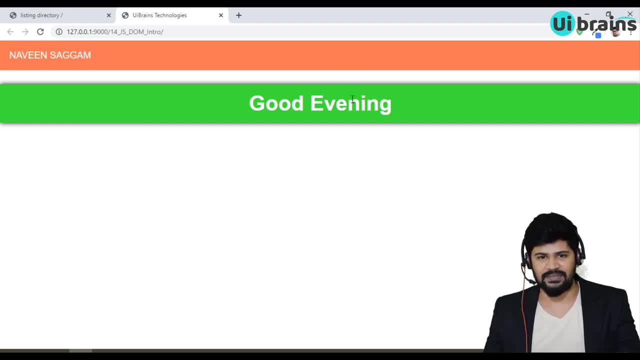 done okay. So for what you want to make dynamic? for what purpose you want to make dynamic? Generally, how you can expect where you can expect the dynamic nature is suppose when you click on a button. okay, do something. So when I click on a button, change the content when. 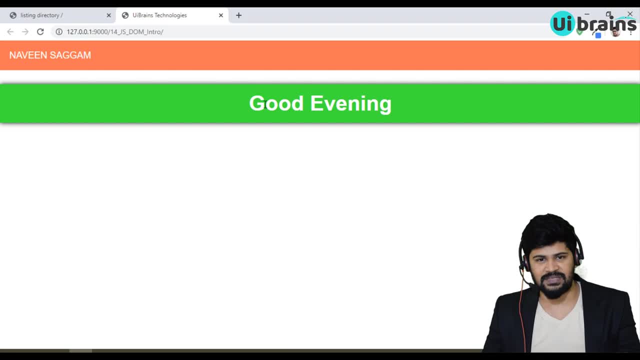 you click on a button, change the text. when you hover on a button, do something when you submit the form- okay. When you enter a URL. okay. when you drag something, when you drop something, when you copy something. 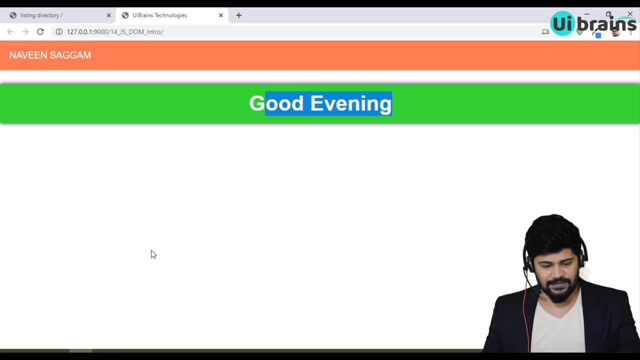 So these are all actually right. Okay, So what is called events? Generally? what is called event is any action which a user can perform on the browser is called event, okay, So any action, you can take, any action. So when you click on a button, right, it is an action. When you enter something in URL. 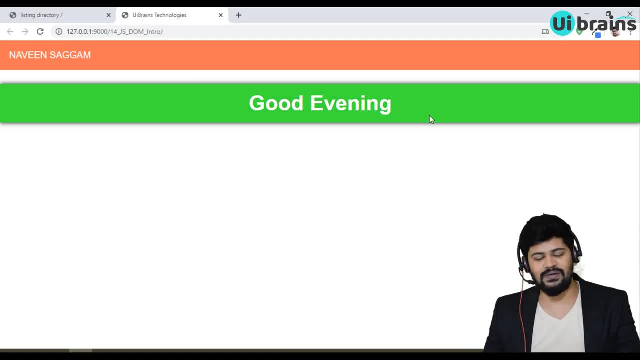 it is an action. And when you copy something, it is an action. So all these actions- there are some 80 plus actions that are available for your document. okay, So for those type of actions, I want to do something dynamic whenever those action. 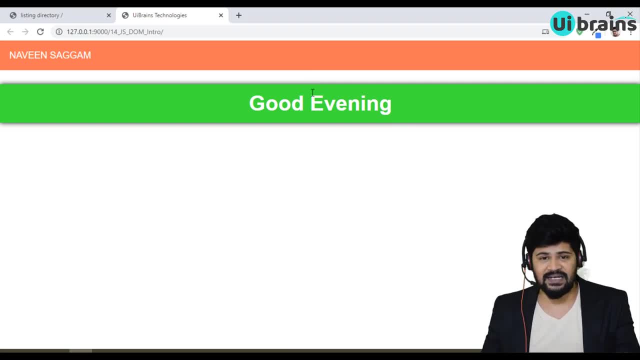 is performed. That's called event handling. So that's where dynamic nature of your application comes. Okay. So first of all, let's understand, sir, what are the actions can be done? Okay, So that action is nothing but an event. So what type of events are there and how to handle? 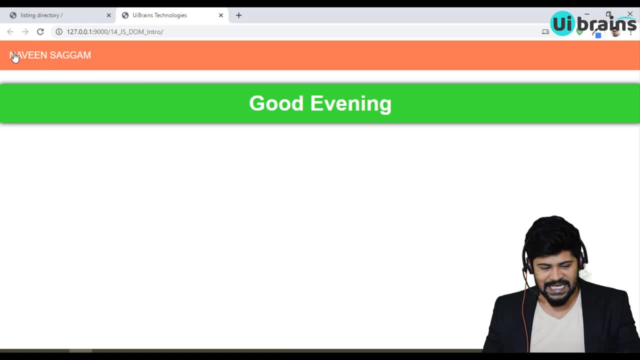 those events. Let's see here. You know any action you perform on the browser is called event, right? so where these events stores all these events you are performing on a browser. so browser represents one object called window object. so in window object there are some events has been written. 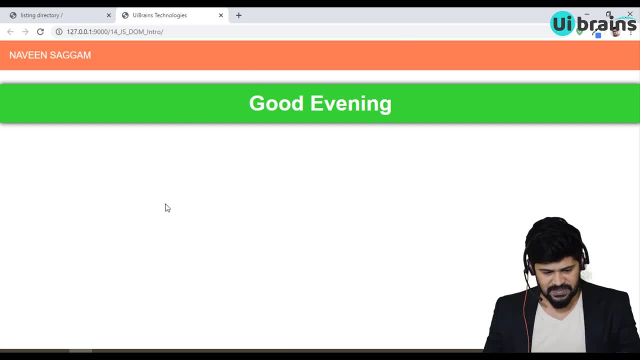 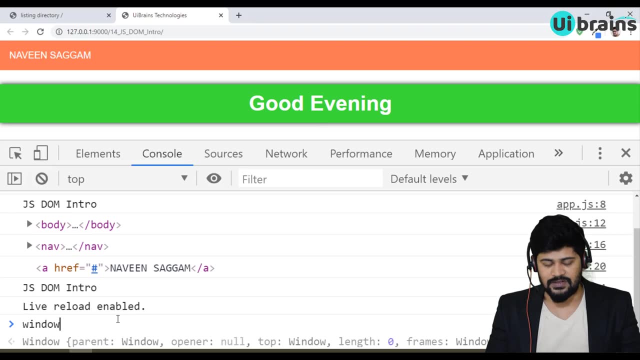 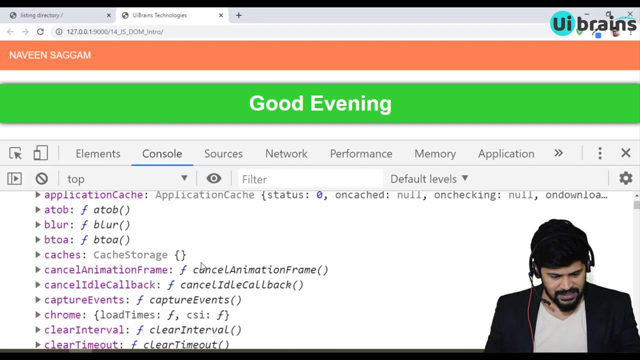 so let's see what is that. let me inspect console. in the console i type like this: window window represent the whole browser. just press enter. okay, so you got the whole window object. so window object represents the whole browser. inside you can find some. yeah, there's something. 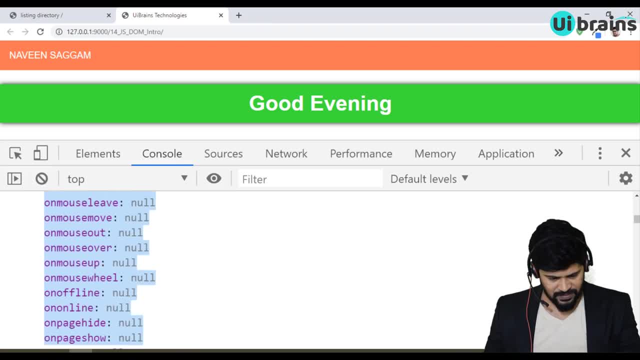 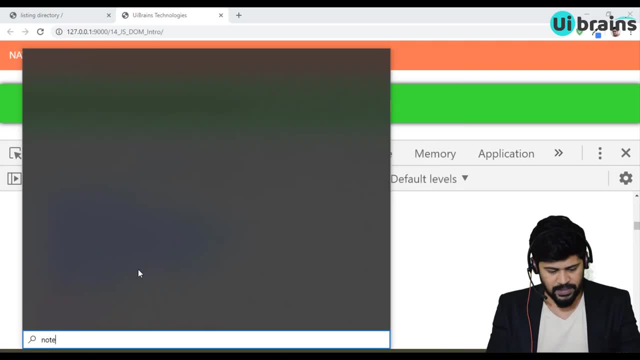 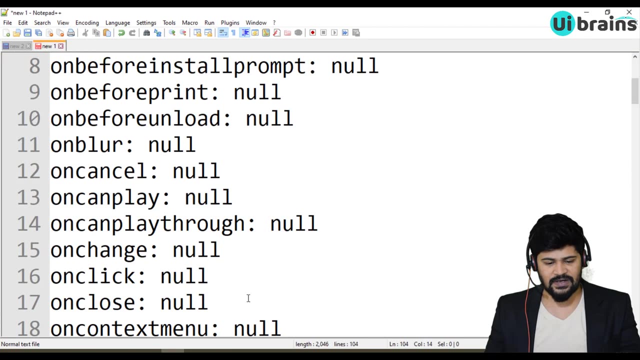 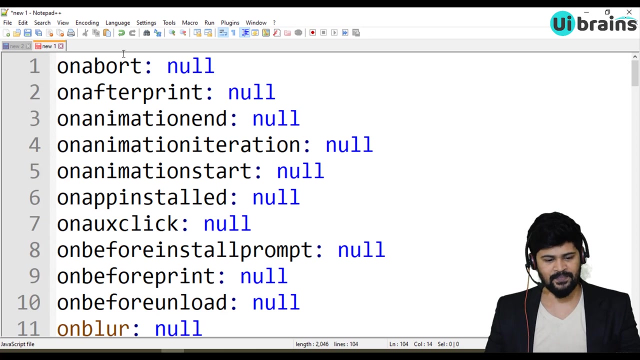 starts from on. so from here you copy everything. yeah, let me copy all this. let me open a notepad, i'll paste it. see 104 events. so these are all actually called events. these are all events of you know javascript. let me change to javascript language. yeah, uh, you can see them on about. on about means, uh, something which is 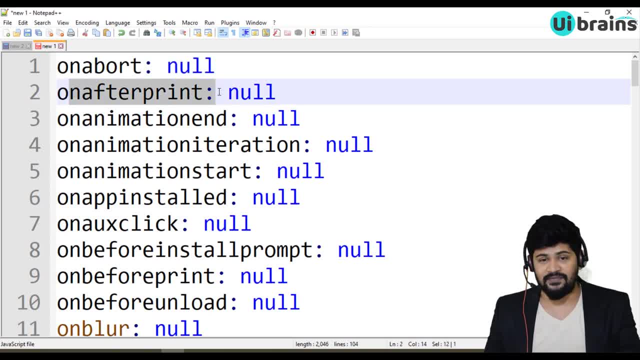 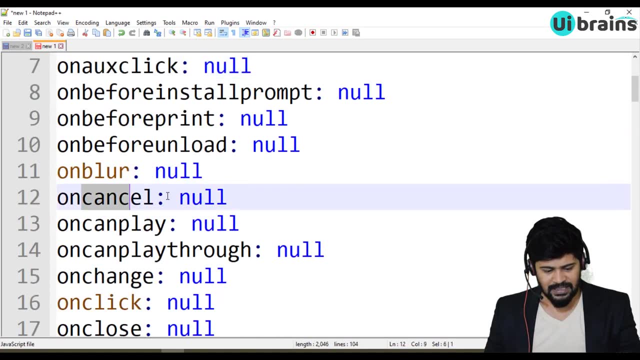 closed unexpectedly. that's called on a bot on after printer. so when you print a document and after that what you have to do on animation end in the end of animation and animation iteration. animation starts aux click on blur, on cancel, on play, on change: when you change something in a 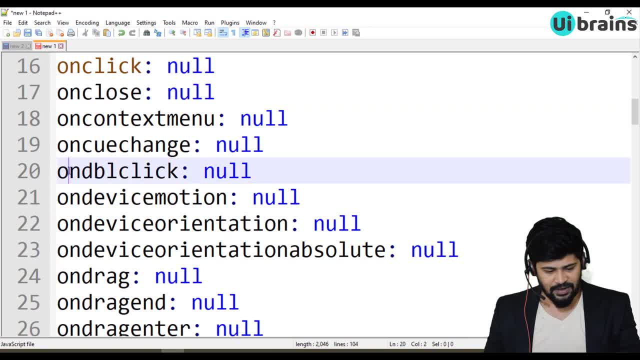 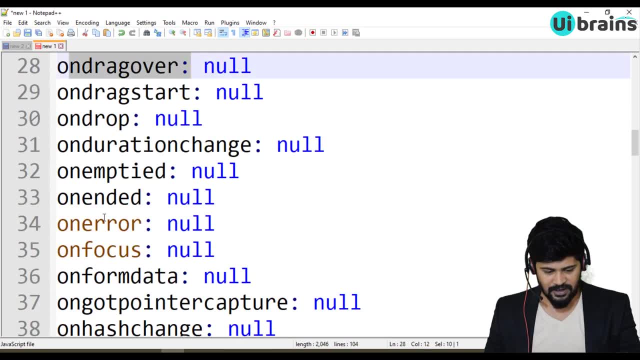 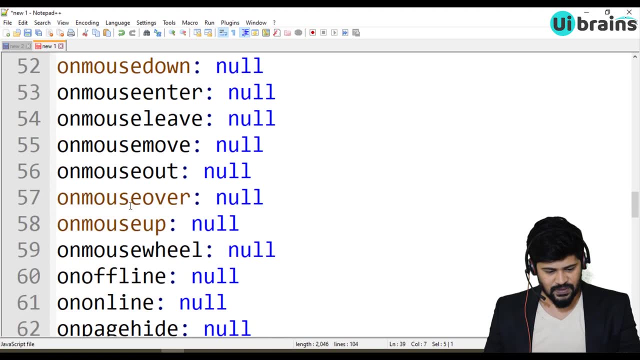 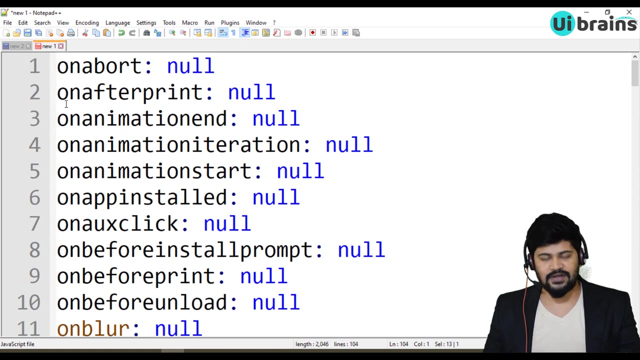 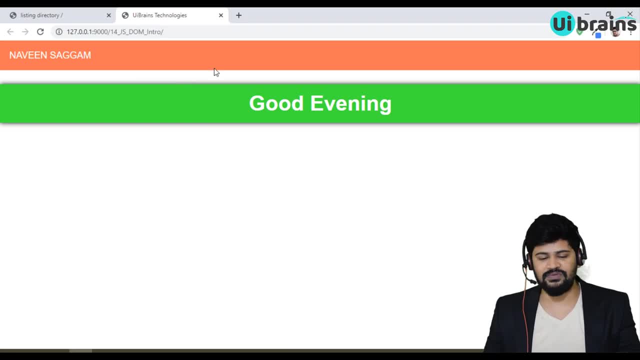 change something dynamically on the page. so how this dynamic thing will be happen is because of these events. so whenever a user is performed an event, then i want to change something on a page. that's how you can really feel the event handling. okay, so that's how you can really feel the 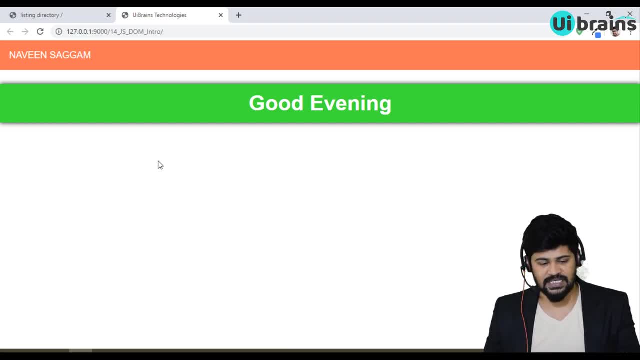 something changing which is on the page called dynamic. okay, uh, let's, let's make an example of some events. what are these is? uh, i'll do one thing. i'll just take some four buttons here, okay, like good morning, good evening and all. so, whatever the button i click, 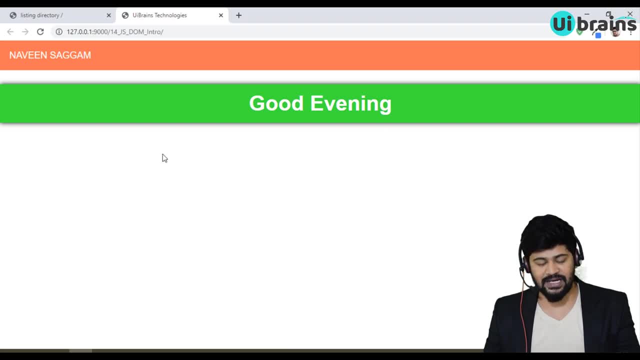 then that message has to be displayed. so if i click on good morning, good morning to be displayed. if i click on good evening, good evening to be displayed, like that. so this cannot be happen with normal html and css. even bootstrap right, so click even will not, will not work. 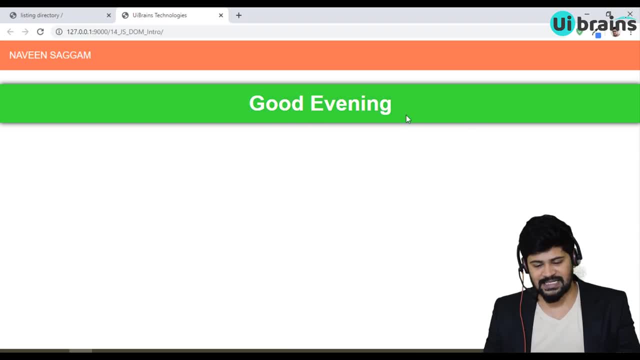 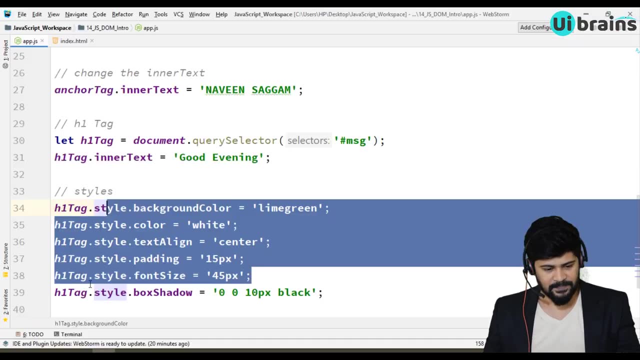 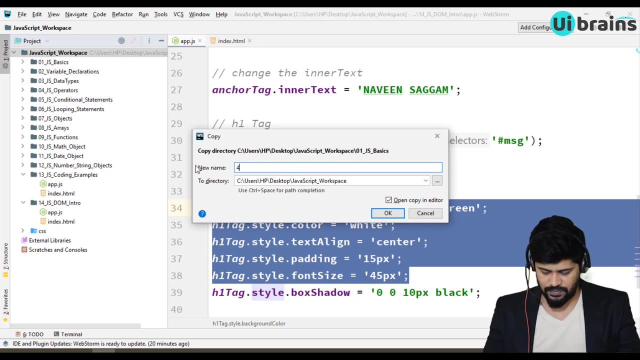 so this only work with dom manipulation. so let's, let's understand. uh, how can you change that um text using the button click? okay, so i'll do one thing. i will just copy the folder, first one, i'll paste it. i change this to 14. underscore: js. underscore: dom manipulation. uh, already there. 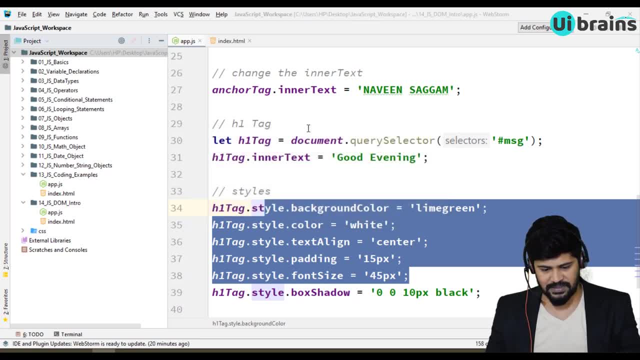 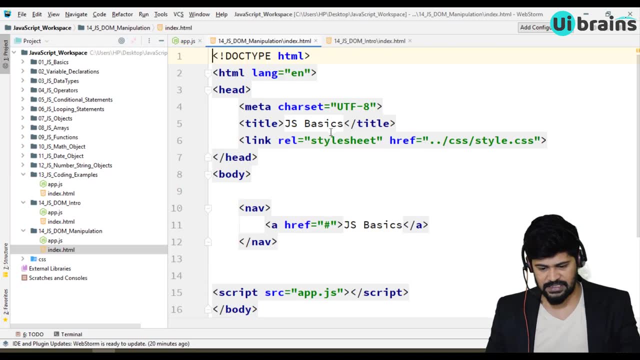 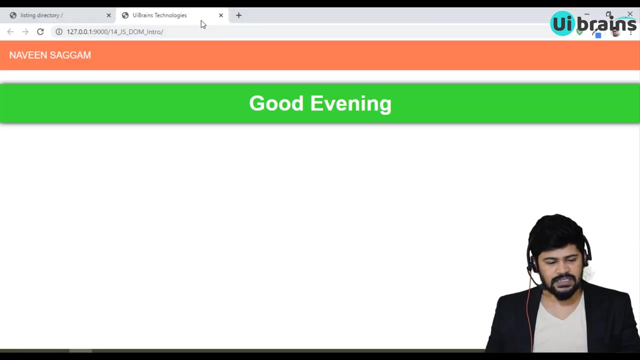 right, uh, okay, dom intro. was there dom manipulation? okay, uh, i don't need this. and then, uh, i'll change to dom manipulation and here also dom manipulation. so let me open this in the browser, close this, refresh um here. yeah, i got it. uh, we don't need actually the console log as of now. 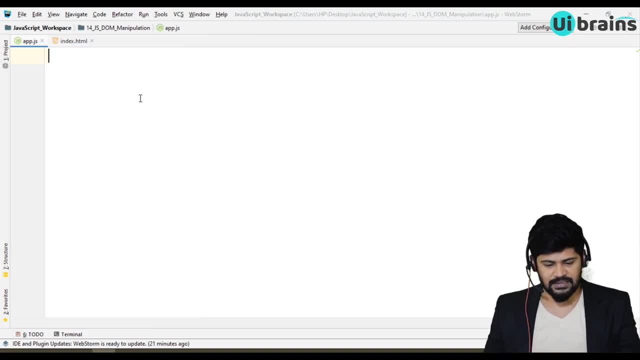 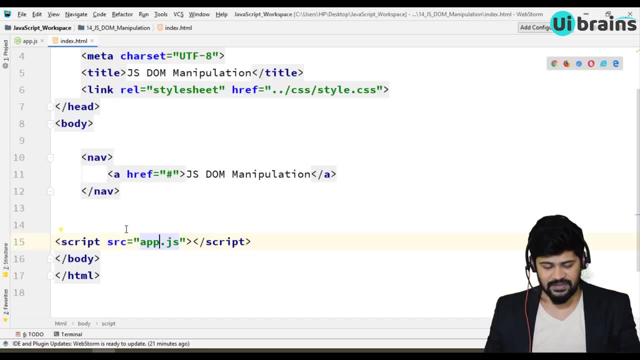 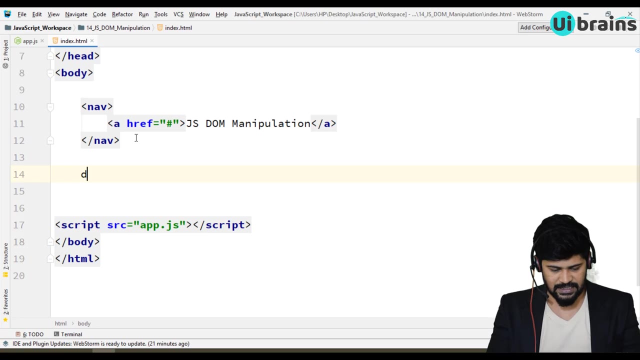 uh, yeah, let me open android js here. let's make some setup. okay, so we need to have a h1 tag and sub buttons texture. so let's make some setup and then we'll start with dom manipulation. uh, so what i do is i just write some some division. i write: 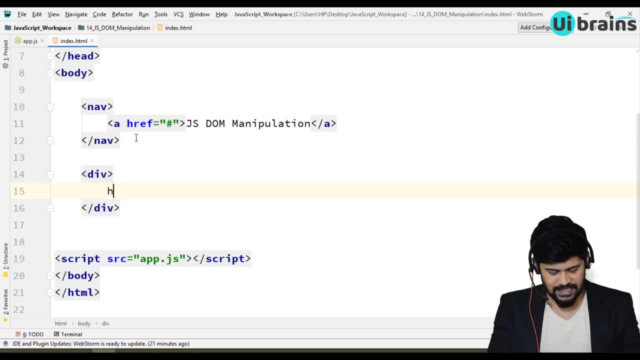 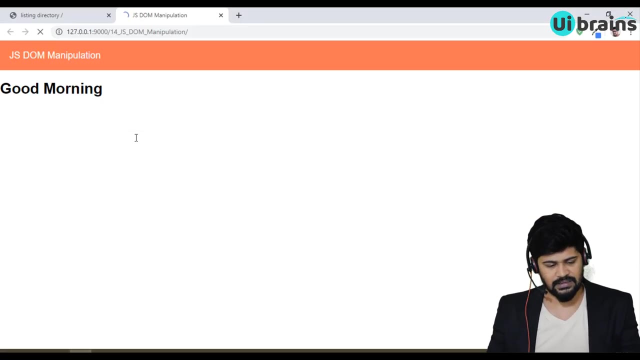 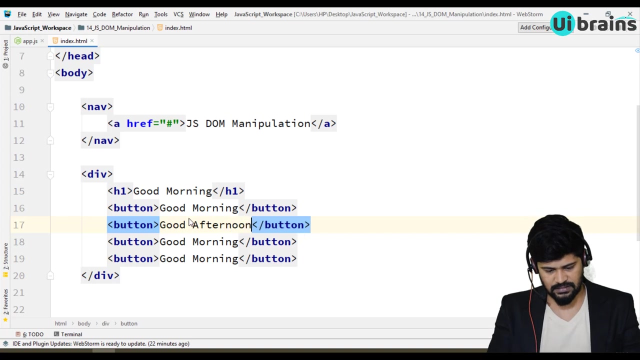 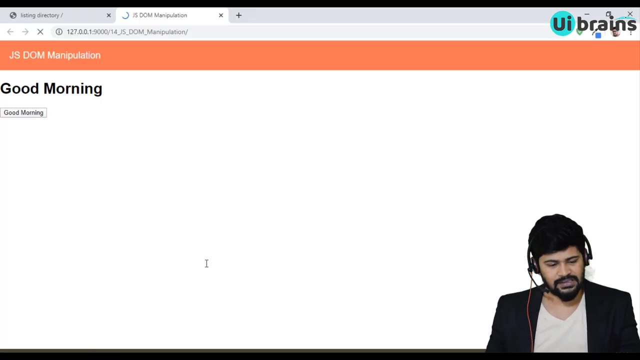 division, division. inside i write h1 tag, something called good morning, i return, and then below that i write some buttons, so button with good morning. so good morning, good afternoon, good evening, good night, good afternoon, this is good evening and this is good night. okay, fine, uh. so let me write some basic styles, also for the background color and something. 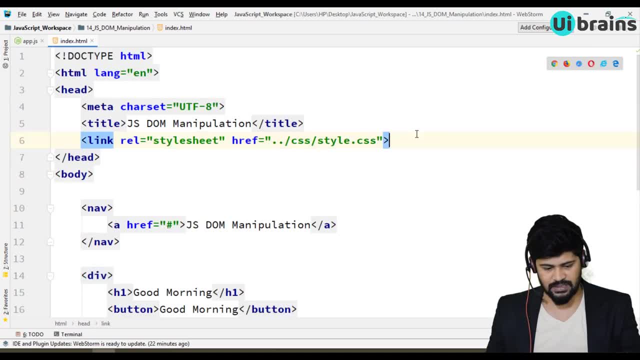 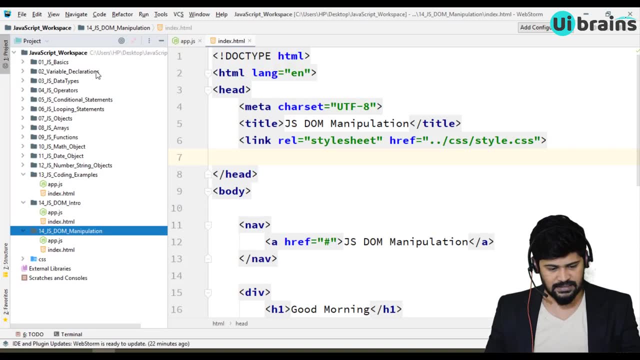 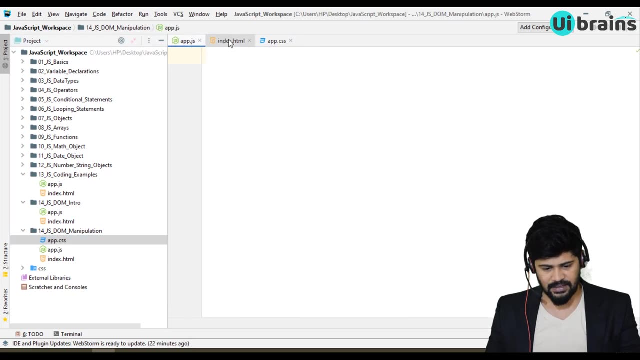 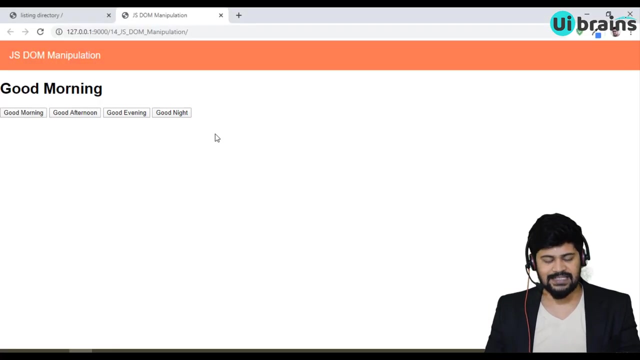 uh, i just take a division, i go to this my own, i write a style tag or i'll do one thing: i create a separate stylecss for this project, this folder, only new style sheet. let's make some appcss and let me connect appcss. okay, looks good. i just want to add some basic styles. 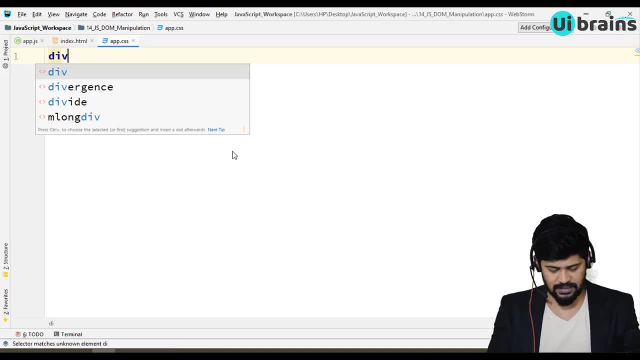 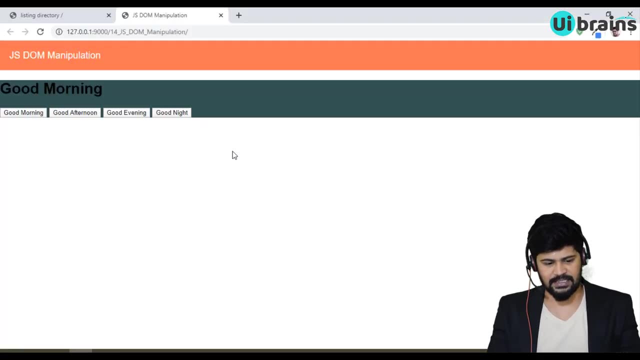 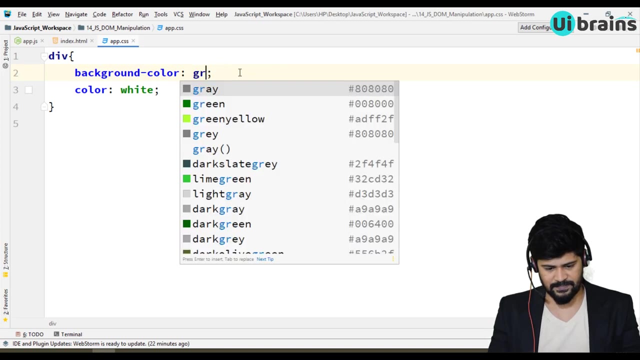 let me give some, uh, division, division. let me give some background color, some dark slits, gray color, and the color i want to be white, not dark grey. let's make some gray color. okay, let me keep it centered, everything, so text align center and let me give some space. that's a padding, padding, some 15 pixels, and, uh, let me give. 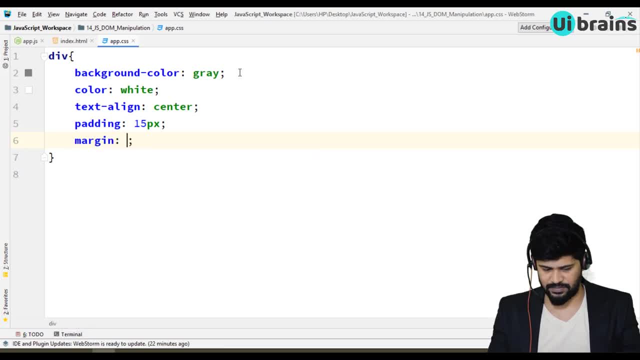 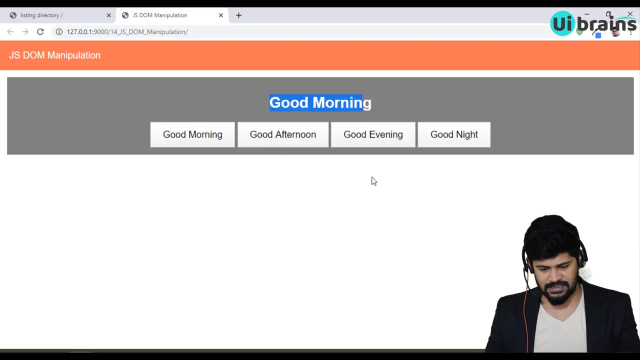 some margin, margin also around some 15 pixels, fine, uh, so buttons, i'll add something. so button, a font size around some 20 pixels and some padding. I'll write. so padding, some 10 or 14 pixels and 25 pixels. okay, fine, but good morning is very less font size. 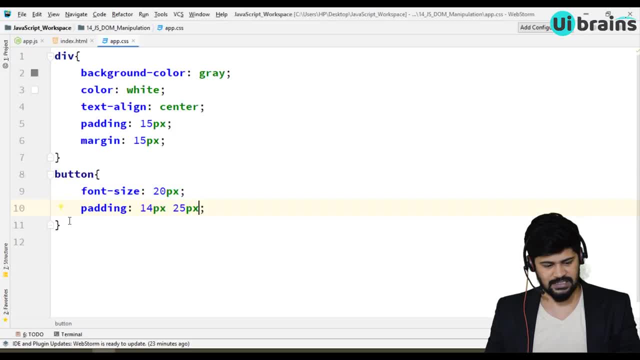 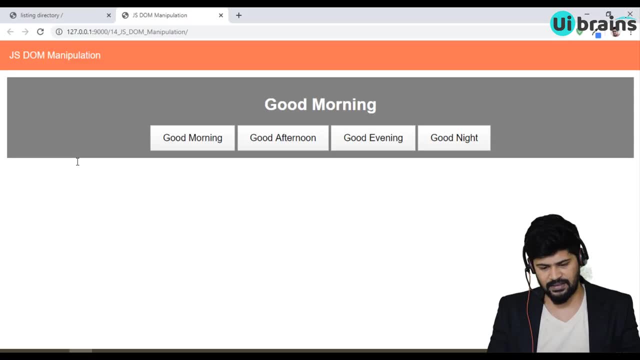 okay, I want this also, the more font size. so I write h1 font size around the 35 pixels less. okay, fine, yeah, so we had a basic setup of html and css. now html buttons you made and css styles you have made, but when you click on any button, nothing happens. okay. 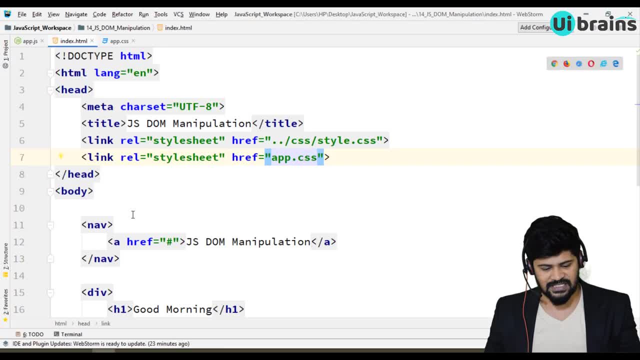 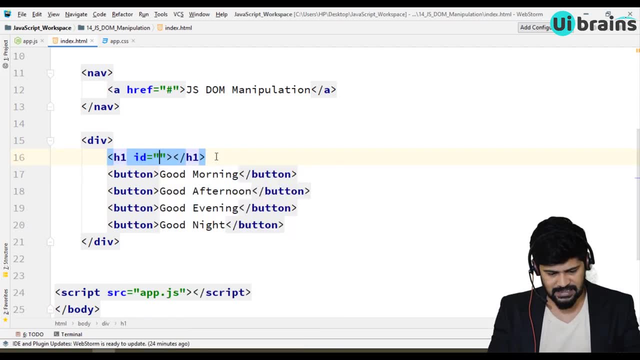 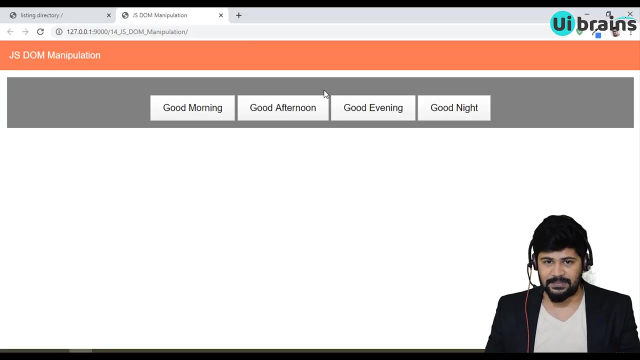 so let's, let's make something over here. so first of all see, I don't want to write anything in good morning, I write some id for this, msg-1. okay, message one. you can, you can feel message one. so if I don't write anything, nothing has display. okay, so fine, I want to display this data from javascript. it means: 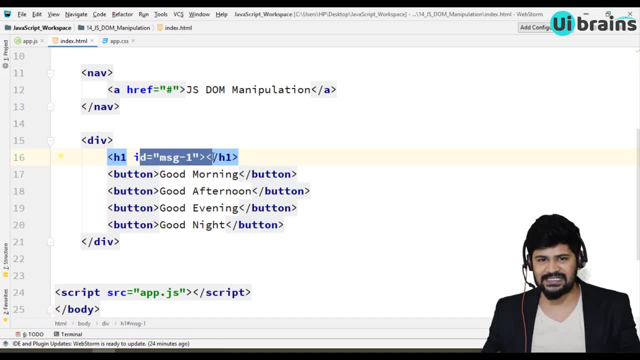 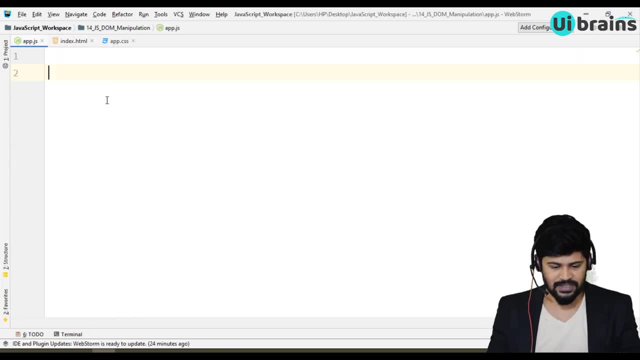 you have to get the id message one and you have to add some extra- you know logic- to display something over here. so let me go to the appjs, tell me how to get the h1 tag. h1 tag is having so copy. so I write: let h1 tag is equal to how you write document dot query selector. let's remember. 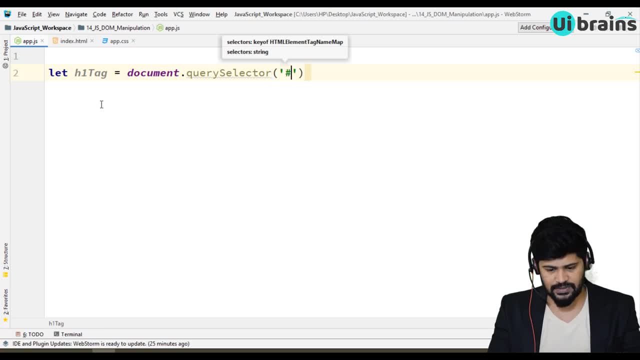 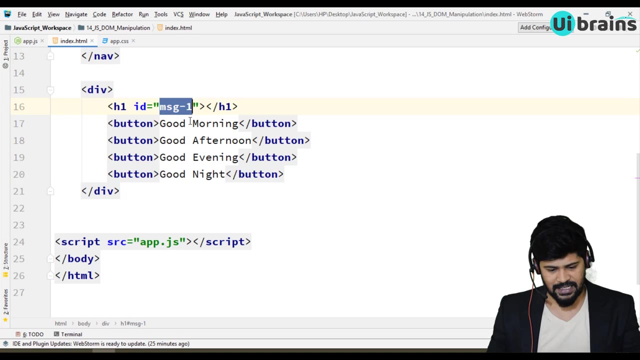 only one function query selector. if it is an id, you use hash class dot and tag is normal tag only. so let's make message one is an id, right? okay, you have an id, so I write hash, fine. next I want to add a texture between the h1 tags. 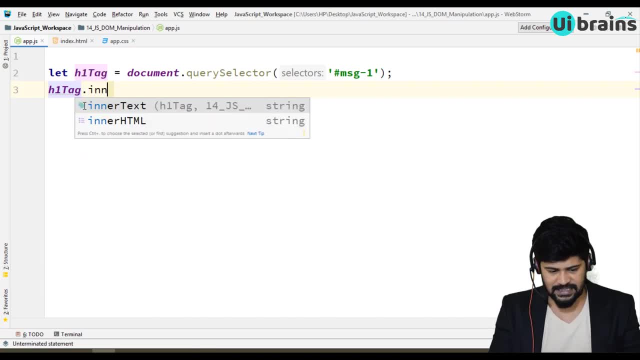 h1 tag dot. that's the inner text. right, the text between the tags. inner text is equal to: I have added good morning. I have added good morning and I do one more thing. I don't want to just write like this. I want to keep this logic inside a function and then I'll call a function. okay, so I'll just 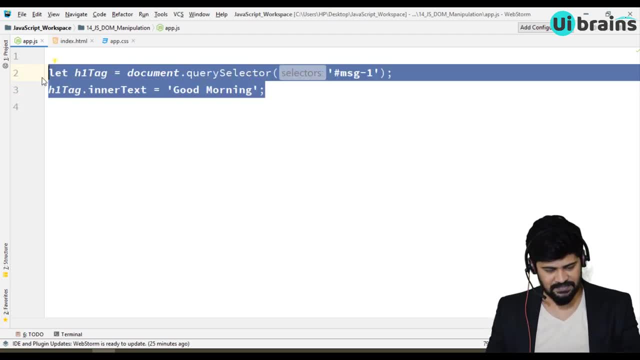 do simple thing: I just cut everything. I just keep this inside a function. okay, let's say good morning. say good morning is equal to one function. you can take normal function like this, or you can take an arrow function. okay, it's a function. I write a logic. it will not execute. 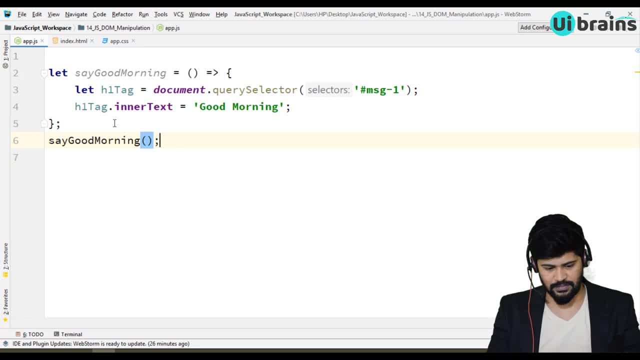 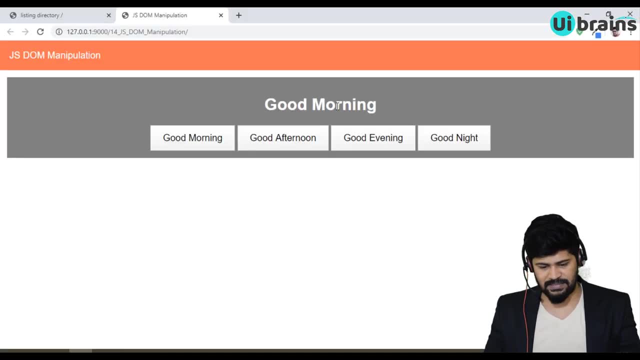 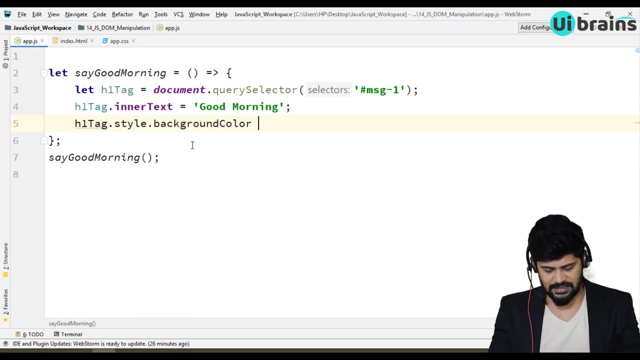 because you're not call a function. so I say, say, good morning, I'll call. okay, fine, now what do you want? I want to give some nice background color. so how you write h1 tag dot, style, style, dot. background color is equal to something called lime green. 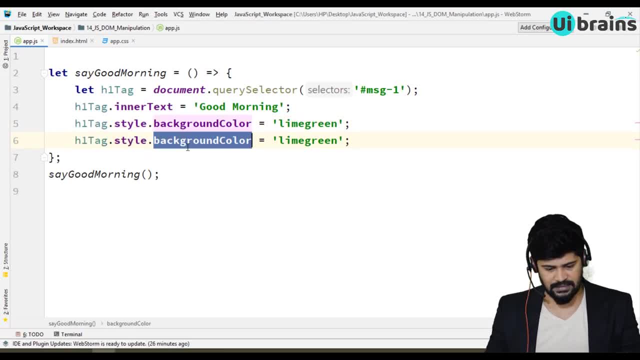 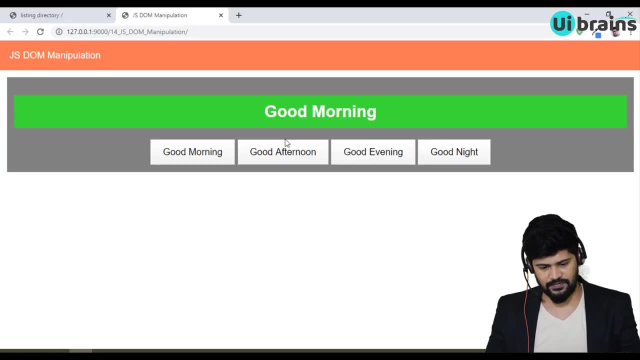 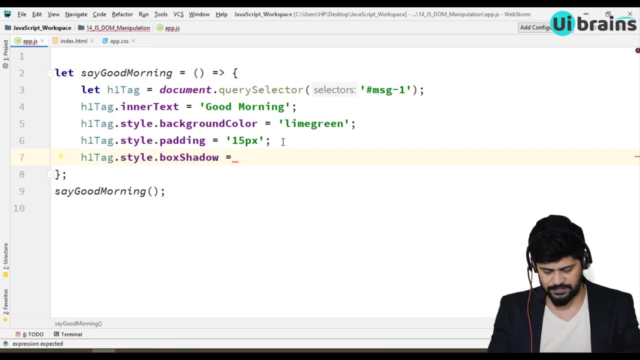 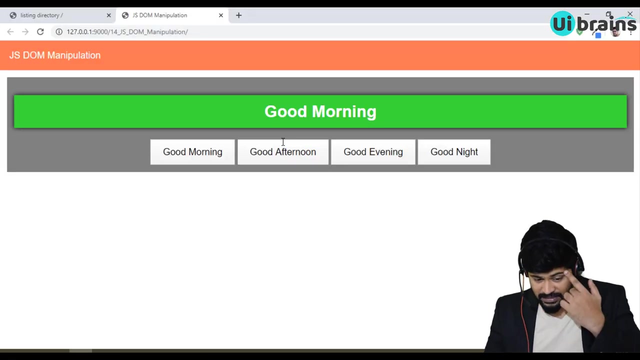 right, okay, let me give some padding. so padding, I write some 15 pixels. okay fine, I write some box shadow h1 tag, dot style, dot. box shadow um, zero, zero, some 10 pixels and black. okay fine. so now here you got good morning and it just works perfectly as well. fine, uh, but I want. 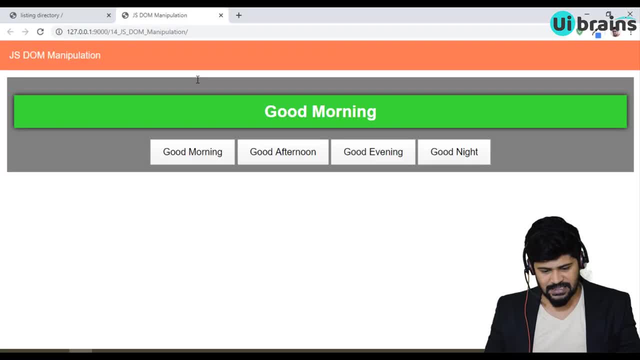 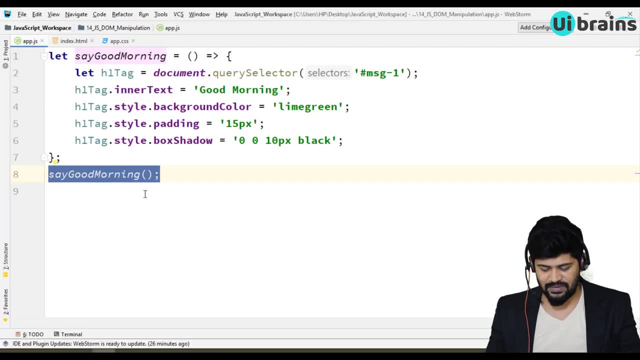 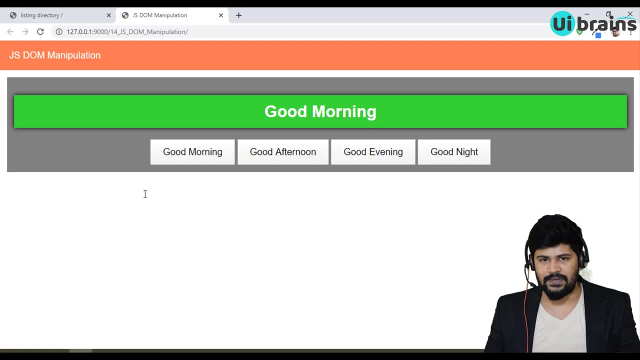 actually the dynamic. what is dynamic, is suppose? uh yeah, you write a function and you call the function. right suppose, if I don't call a function, what happens? nothing will display, okay. so if you call a function, then it will display. nothing will display, okay. so if you call a function, then it will. 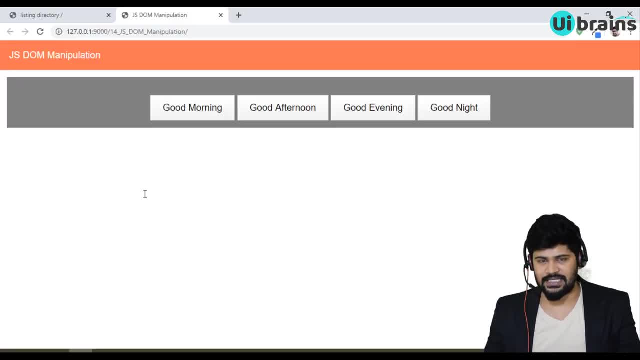 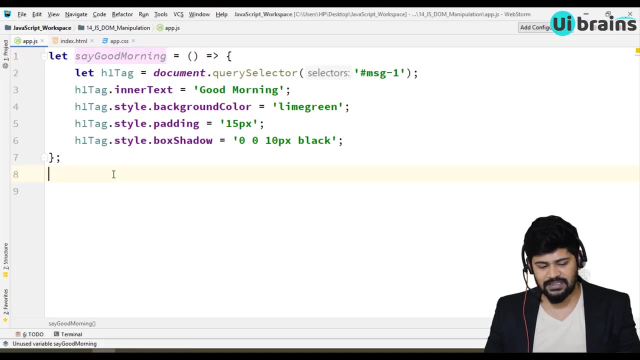 display. if you don't call a function, it will not display. okay, that's one thing. now, actually, when you have to display, when you have to display is the moment when I click on this good morning button. then I have to display, correct, actually, how it is displaying when you call this function. 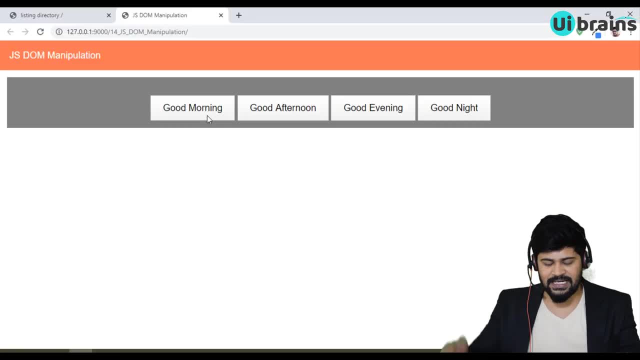 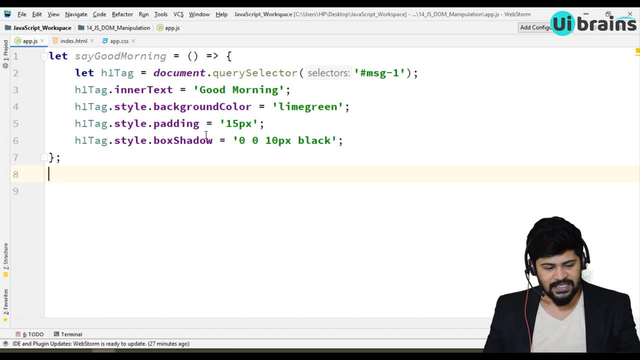 it is displaying, but when to display for us? not immediately, as soon as the page loads right. so the moment I click on this button, then display it means the moment when you click on this button, then call that function, then it will display. so how to call a function when you click on a button is: where is this button? 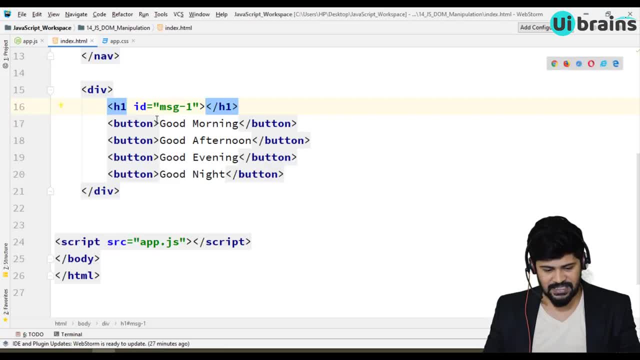 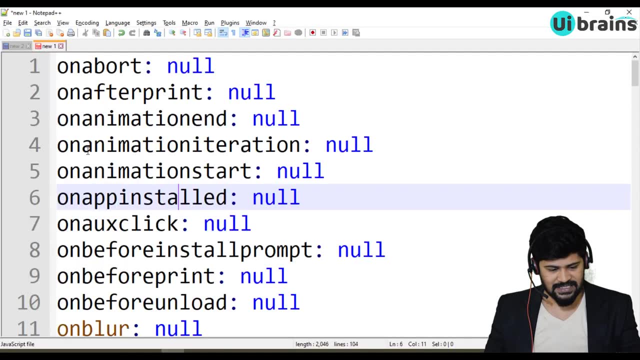 logic. this button logic is inside a h table, see here. uh, so here for the button on click. so we have already seen, uh, the events. right on. there is something called on click. is there? you can find somewhere, I think, on click this event, okay on when you click on a button. so on click the. 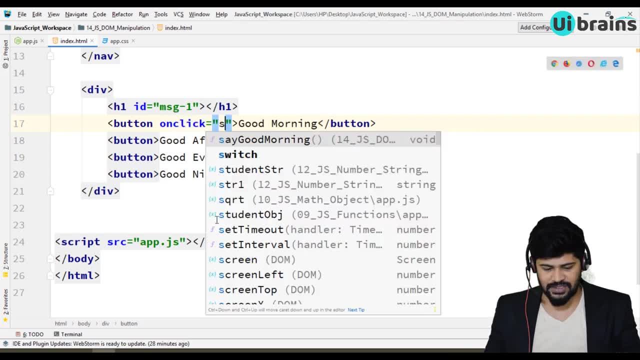 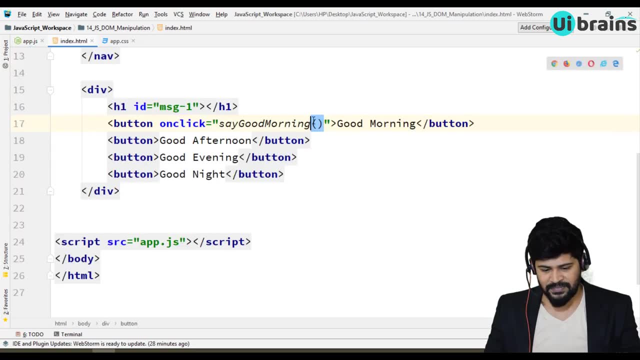 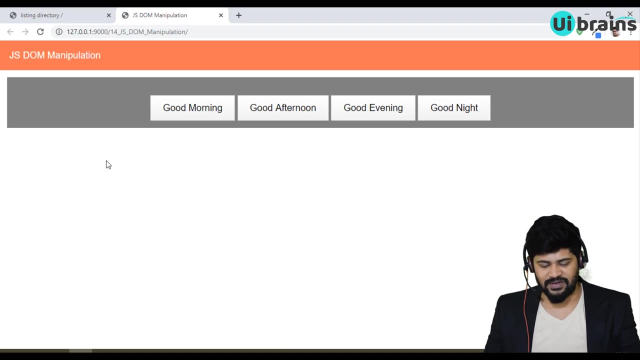 moment, the moment you click on a button, I want to call a function. call, say: good morning. see, I'm not calling the function here, I just write a function. but I'm calling the function the moment you click on the button. now check here, nothing has displayed. okay. so the moment when I click on this particular 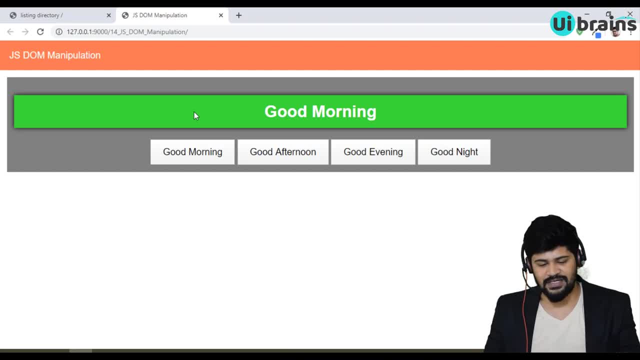 button, then display. so that's how even handling okay. so when you click on a button, you write on click, you call the function and it works fine. so when a page loads, nothing will display the moment when you click on the button then display. so this nature cannot be done using normal html css. it's only be done using a dom. 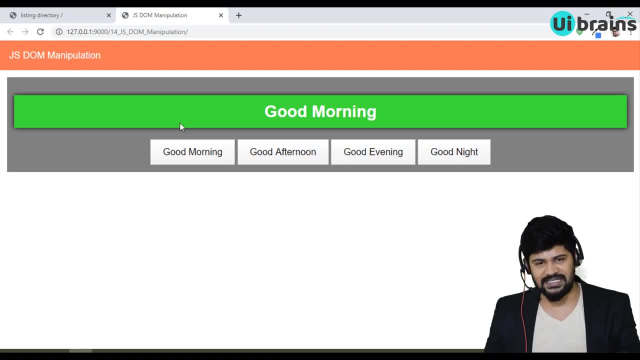 manipulation of javascript. one more thing is pending. what is that is, when I click on good afternoon, I change this text to good afternoon and color. I have to change good evening and good night also. so what you do, good morning. you made a function, so same like that. I'll copy this. I'll. 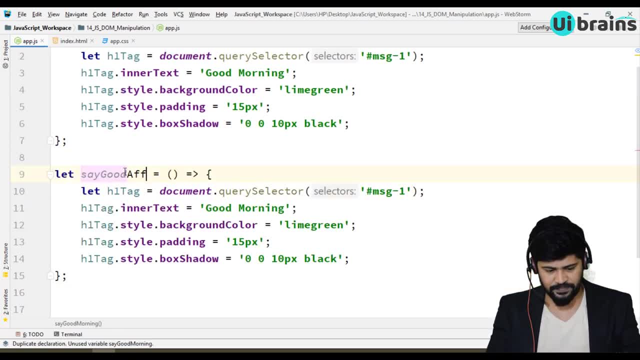 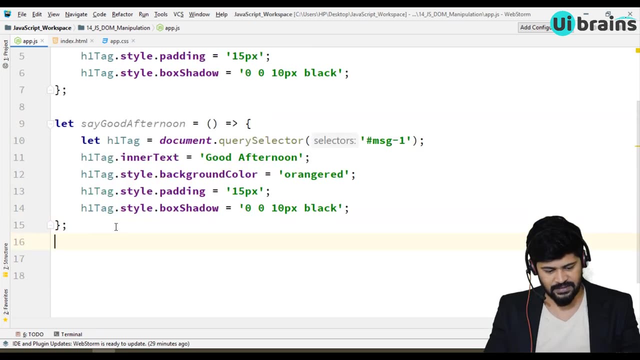 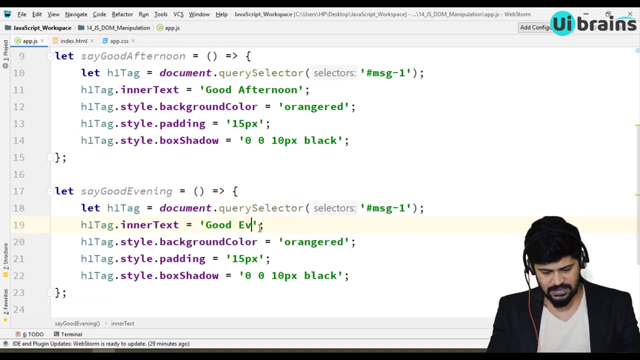 make another function. so let's say: good afternoon, okay, I make it as good afternoon and color: I'll make some orange red. okay, fine, let's call. let's create another one more function for a good evening. good evening, let's make this is also good evening and good evening in purple next. 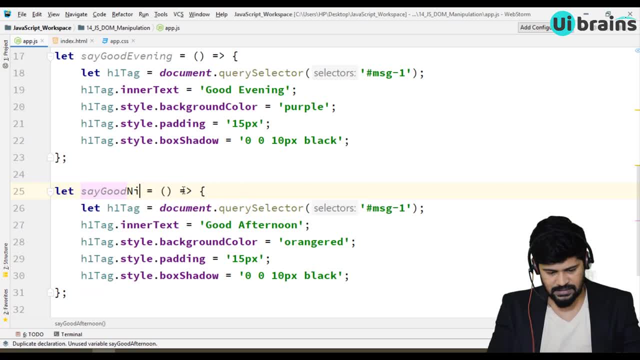 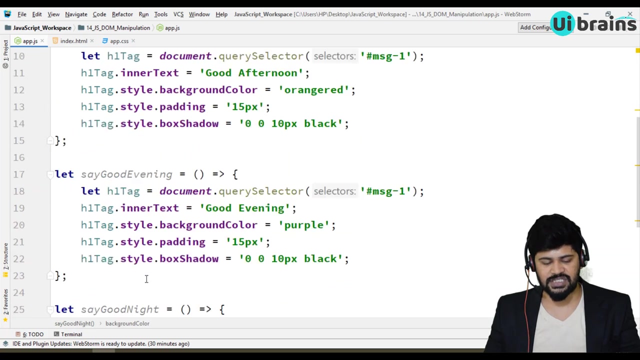 paste it. I want to make it as good night, okay, so this is also good night. and good night is actually: um, what color? blue color, okay. let's take black color, okay, so it's, it's black, fine, uh, so you have made four different functions and call them. so wait to call here. so here, good afternoon on. 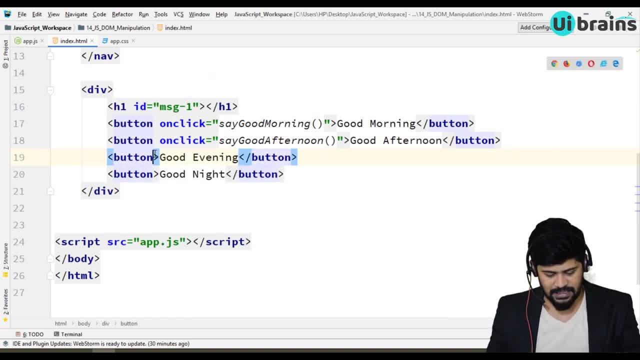 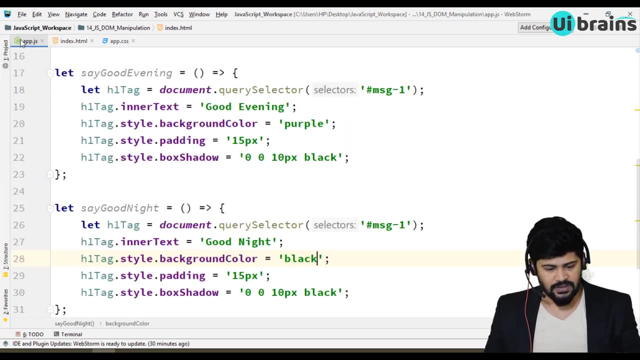 click just say good afternoon, and here, on click is equal to say good evening, on click is equal to say good night. see, I'm writing a lowercase, uppercase, uppercase is a camel case, right, fine. so now see, you have made four different functions. and you have made, you have called. 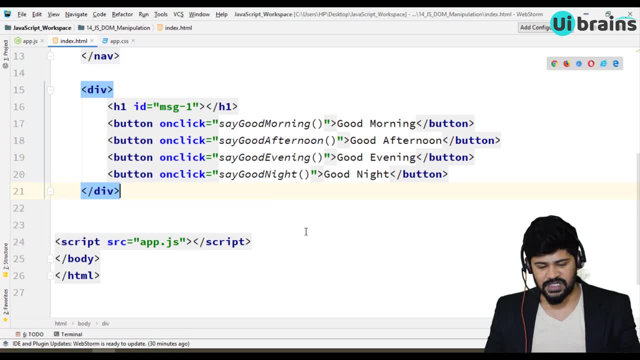 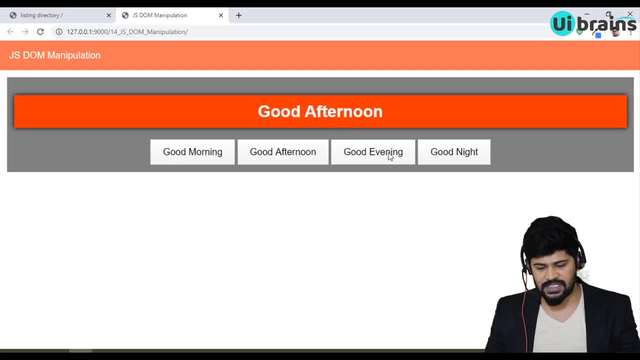 when you click on different buttons, different functions, right now, check, nothing has display. when I click on good morning, good morning: display. when I click on good afternoon: see, it is change. good evening, good night- see. so whatever the button you're clicking, so data has getting changed and its color has getting. 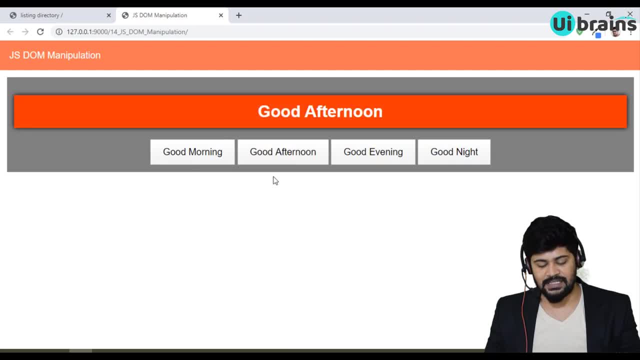 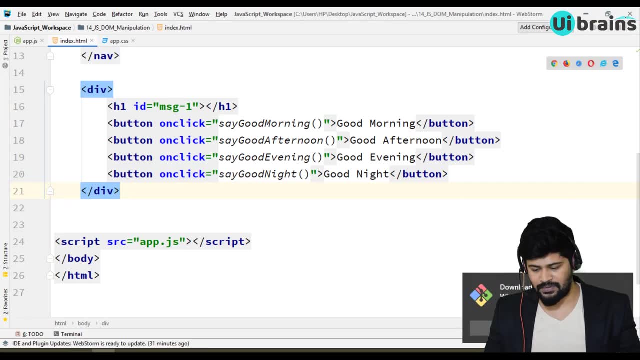 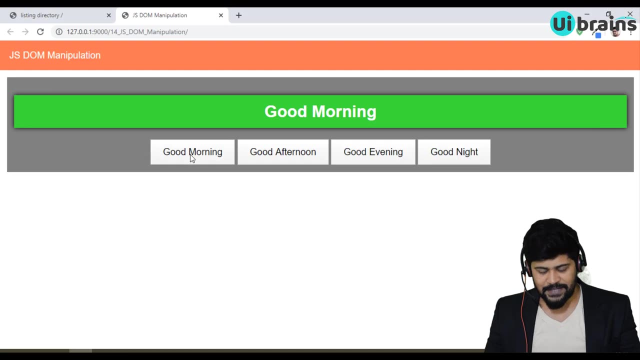 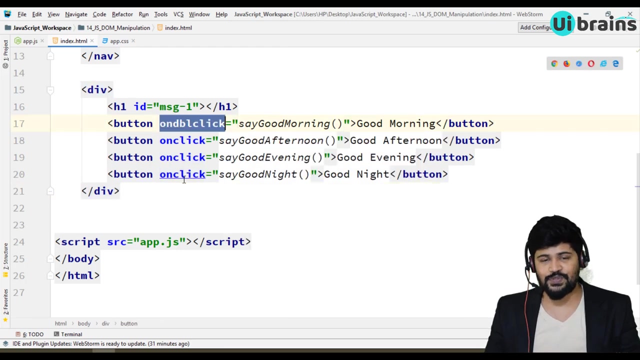 changed. so this is actually a down manipulation and that's this one dynamic, correct? oh fine, uh I. I want to tell you one more thing. I want to tell you one more thing. what is that is on click. when you click, then works right. um, I write something called on dbl, click on dbl. click means what on? 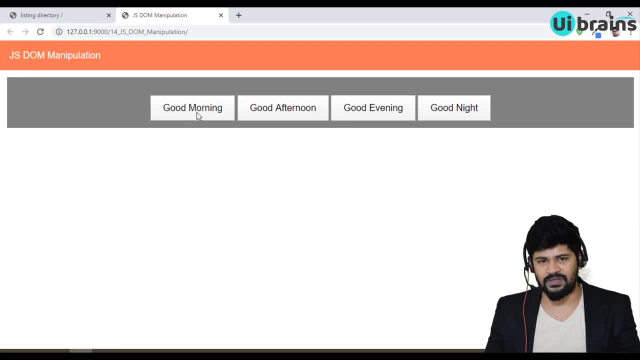 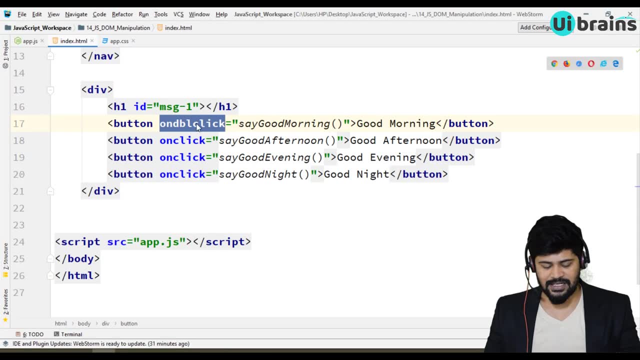 double clicker. so when I click it won't work, because it's not click event. it is what double click event? so when I double click, then works okay. or else you have many things. you have like mouse center. I tell you something called mouse enter. what is mouse enter is, it is not click, it's. 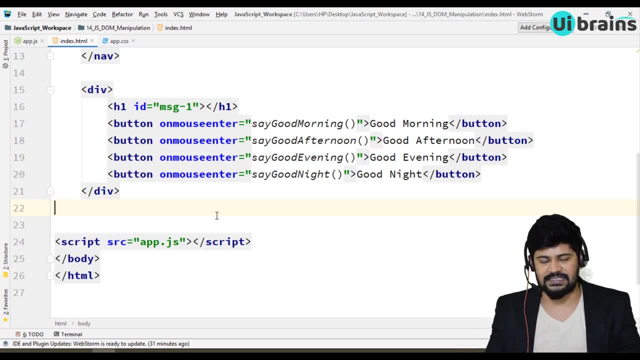 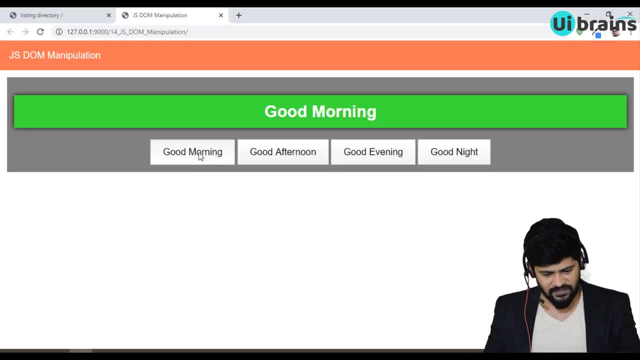 mouse on top of the button. it's an event triggers. okay, just just pass the mouse on top of the button. okay, see here, see I tell you this is called click event. you can feel something. right, I'm not clicking now, I just pass the mouse cursor. see, I'm just passing the mouse and you got data. 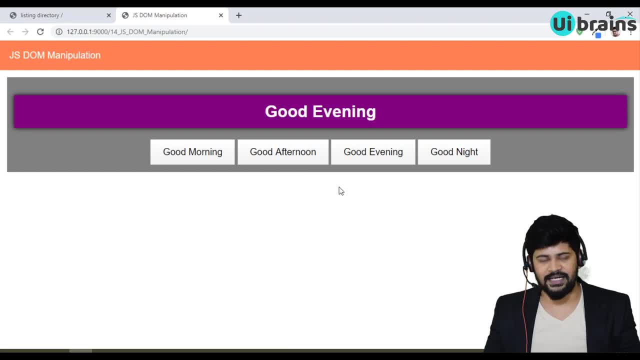 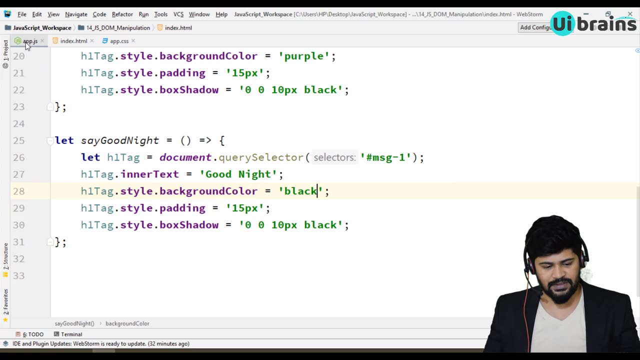 getting changed. okay, so this is called mouse enter. so we'll see this events ladder, but as of now on, click events. okay, so it works perfectly fine. but, as I told, try to write a logic first and then try to optimize the logic. what's most important, okay, in programming? see, here we have written. yes, 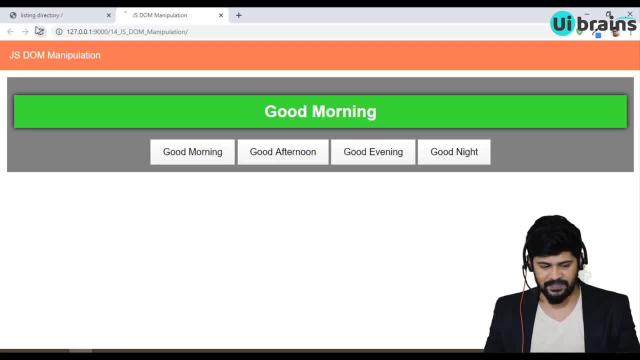 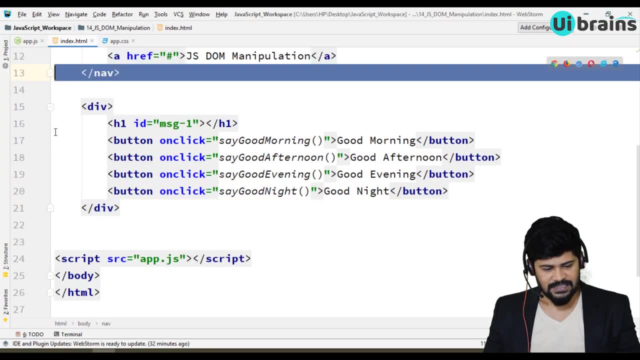 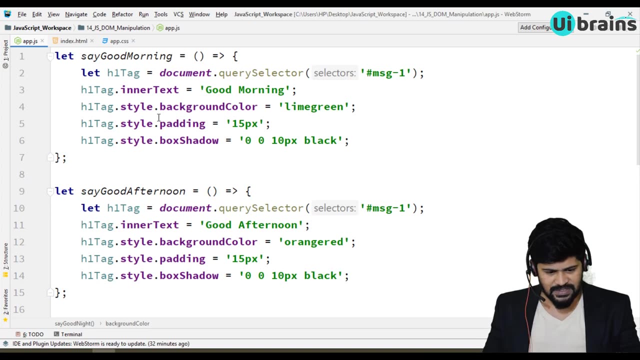 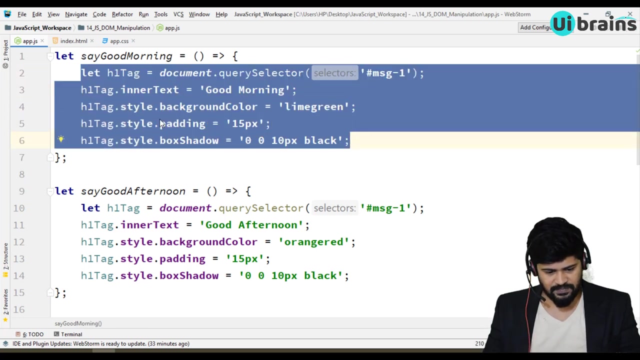 it works down, manipulation works, we are satisfied, fine. but thing is, sir, just change a normal text here. do we really have to write these many lines of code? okay, let's understand what it is. if you observe closely, every function will have same set of code. right, this is having a. you know violence, you also same, it's also same. 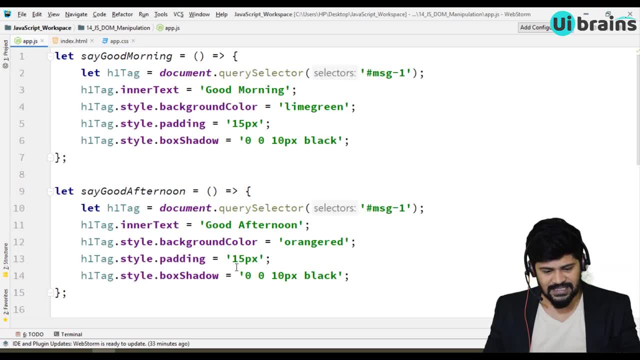 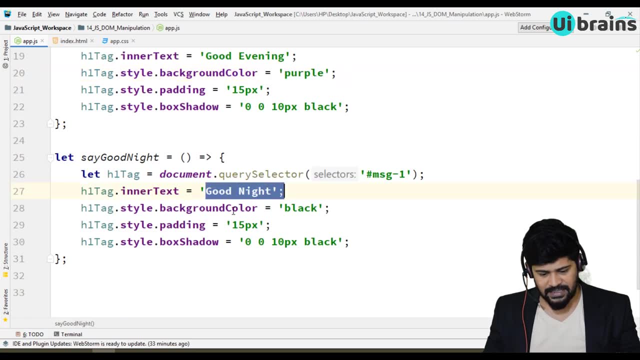 all same, but only something which is different. what is that? is here good morning color, here good afternoon color, here good evening color, here good night color? only just these two lines different. so why can't you pass these two data dynamically to a function, right? so let me optimize this. what? 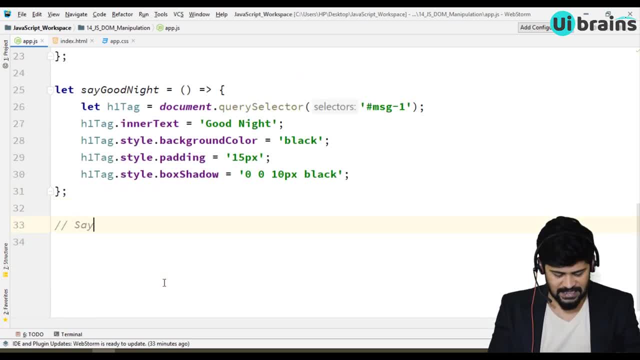 I do is I create a separate function. say let's say wish, wish me. okay, let's make. okay. let's say printer wish message. okay, let's make my own function: print to wish message. you can take any. I said let's print message is equal to: I write an arrow function to get a number function also. 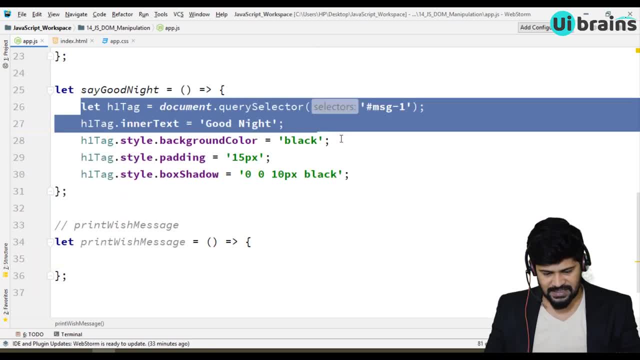 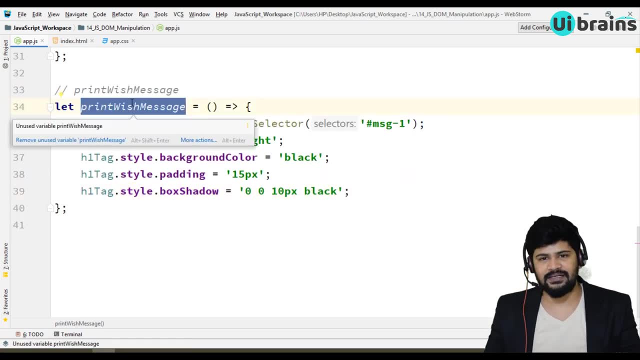 fine, so here I will just copy everything, I will paste it, okay, here. if you call this function, what happened? how many times you call a function? always you get good night and black color. but I want dynamic. so what you do? this dynamic, this dynamic. so what is this? a message, what is this? 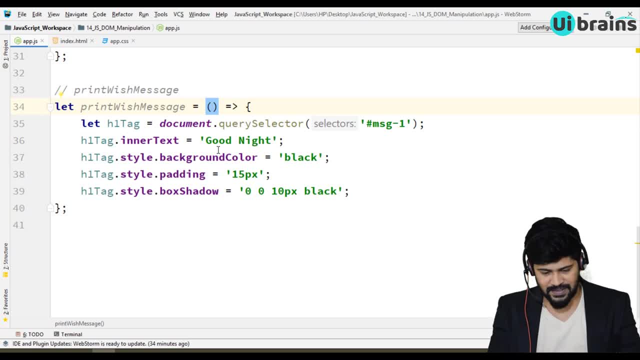 a color. so you can just declare them as the parameters. you can declare like message: comma, color. okay. so if you pass good morning, I want to substitute that good morning as a value here. next, if you pass color, I'll copy that and I'll paste it here. so if you pass white, 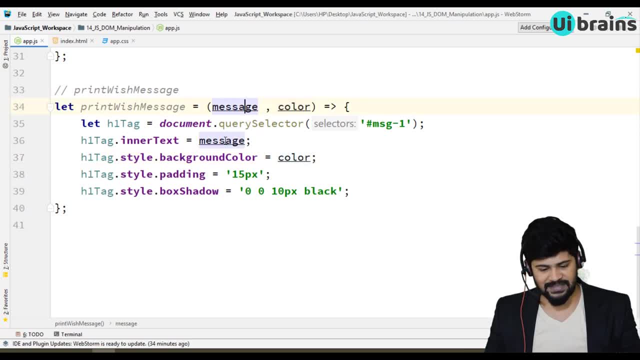 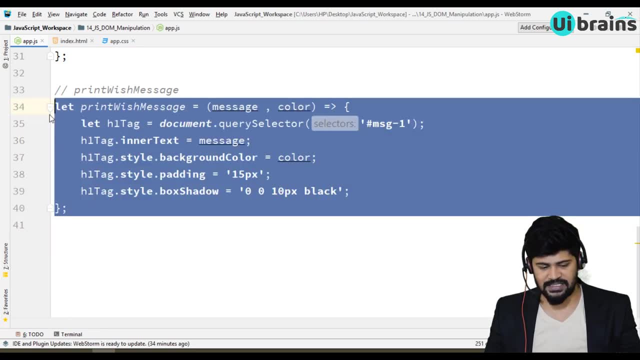 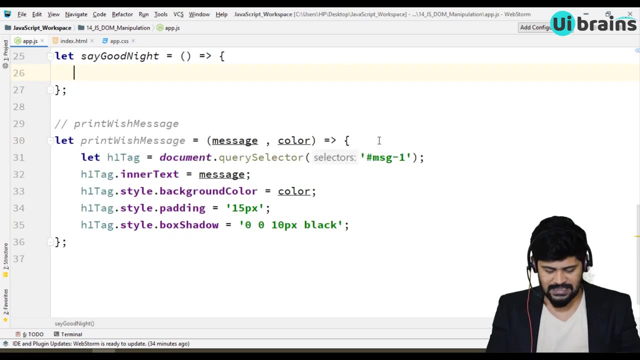 it apply white. if you pass black, it apply black, and even the message. so now we have made a general function, so what you have to do is just call only this function from your file. so what you do is either you cut this print to wish message you can pass. 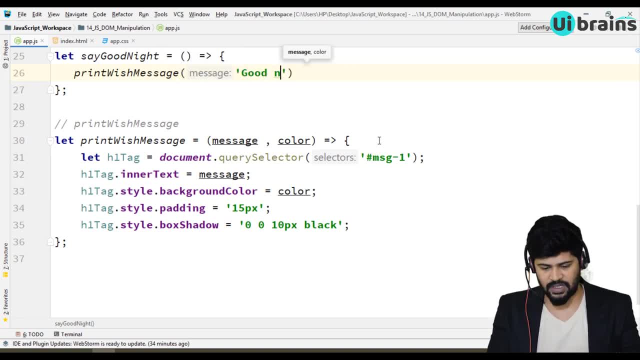 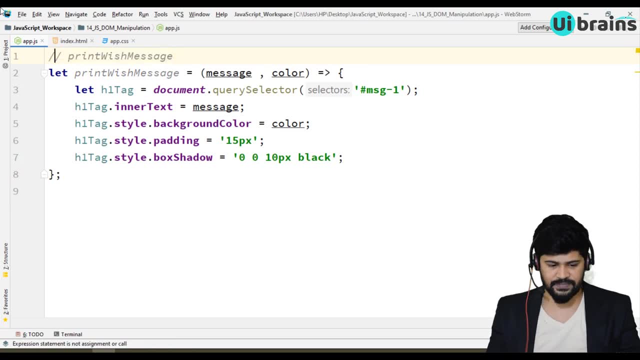 the message called good night. okay, or else I tell you easiest way you can delete all this. okay, not required. you just make only one function print to wish message. only just one function, okay, so this function. I have to call with the message and color. so what I do is: 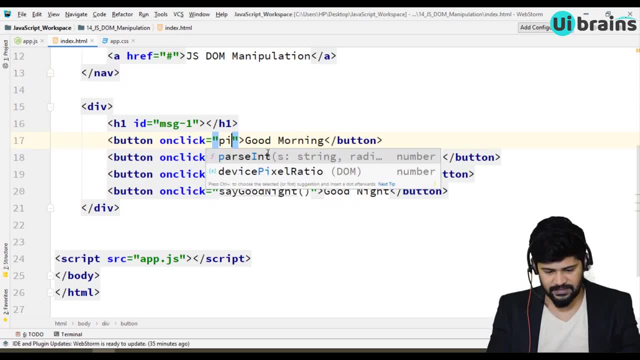 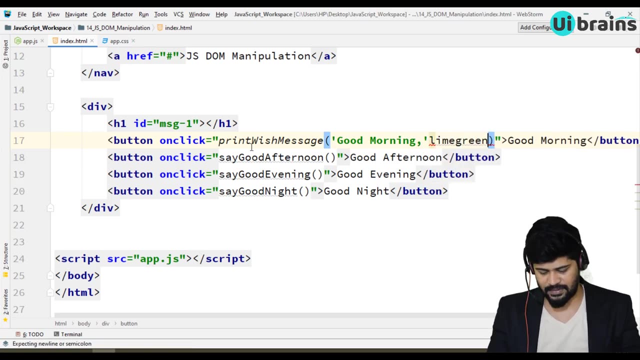 instead of saying good morning printer wish message, it expects what message and color, what message you want. I want good morning, and what color you want? I want lime green. okay, I need to make us good morning. I am green, okay, single course. fine, let me copy the same. 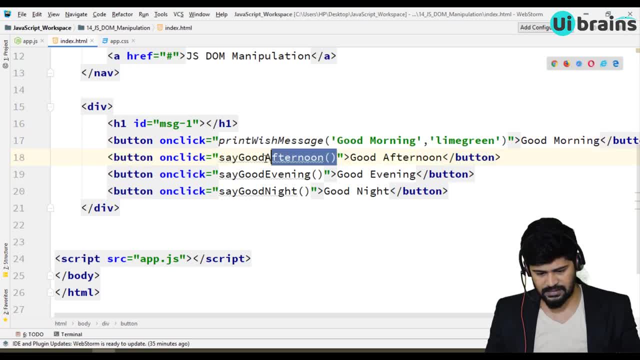 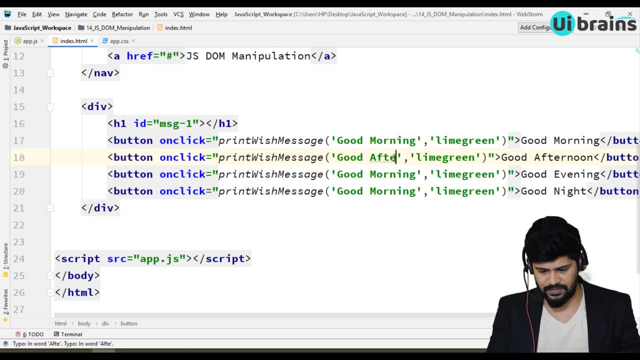 I paste here, and I paste here, and I paste here. so this is going to be what good afternoon. and it was what orange red color. this is good evening, this is a purple, and this is good night, and this is black. that's it. so see, here we don't have any function, we have only one function, and 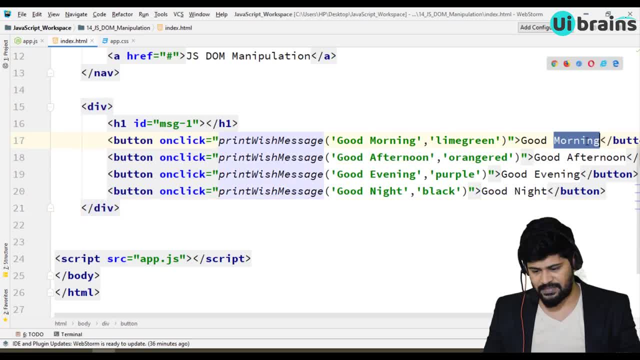 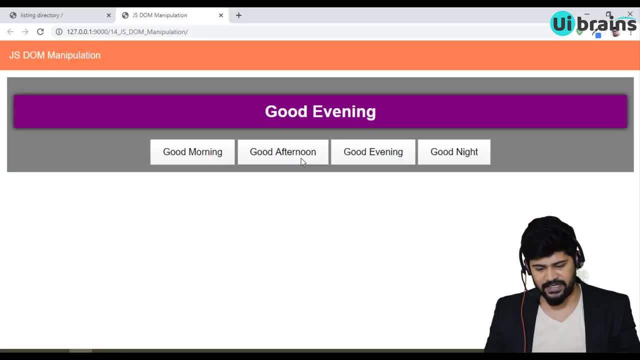 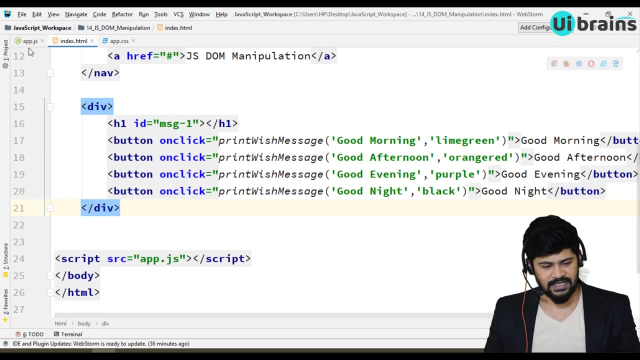 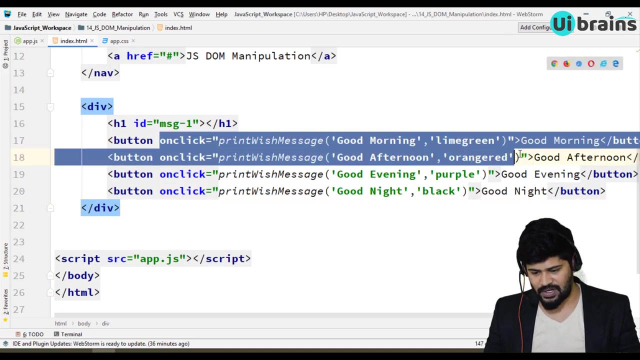 we are calling that function for every button. we are calling the same function but different message you are passing. okay, now check. yes, it perfectly works, correct. so this perfectly works with the very less number of lines. okay, and one more thing here is: we have made a function call. 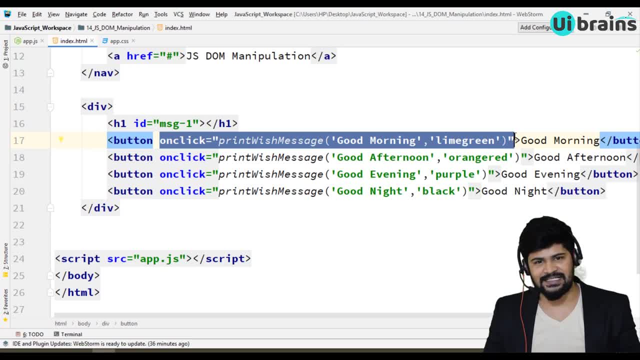 in HTML. one small limitation here is: we have made a function call here. actually, you are not supposed to add a function call here. I tell you without writing on click in HTML, how this functionality make it works. okay, so that will tell you in the next video. thank you so.